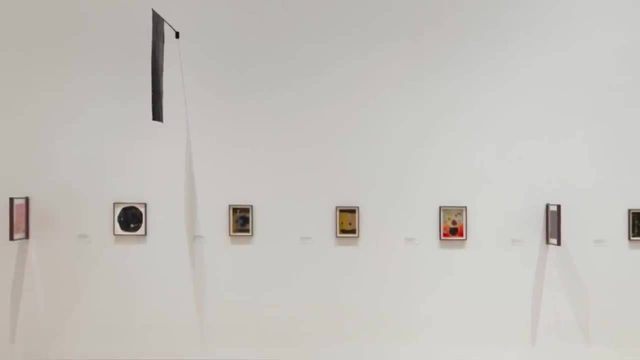 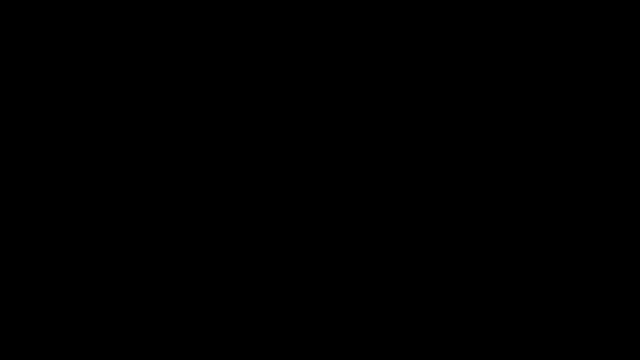 found objects. We are eager to discover what 2022 will bring. Gabrielle Liron-Del-Hill, and what the artist will bring to 2022.. Number two, Ritzit Gobben. One of the lesser-known artists from our list. a true discovery in 2021. 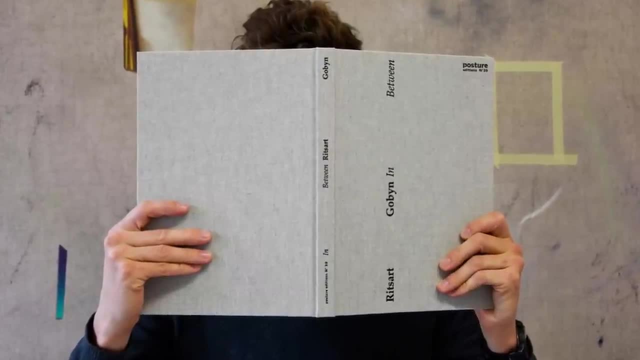 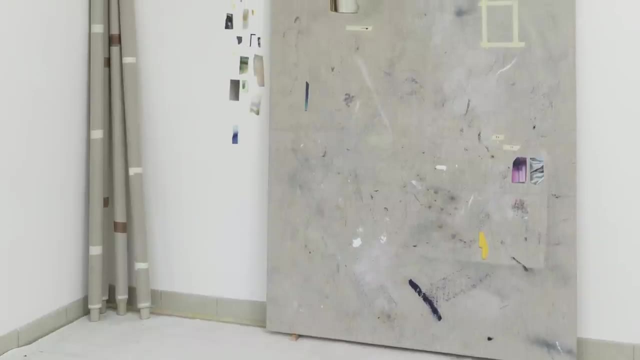 is one of Belgium's most promising young artists: Ritzit Gobben. Born in 1985, Gobben lives and works in Ghent and is best known for his unique Tromp-Loy paintings marked by subtlety and 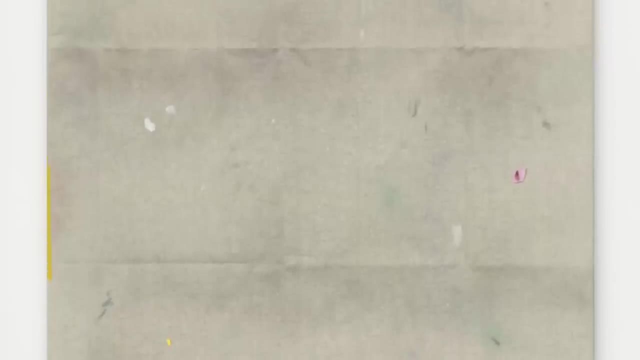 illusion. At first, Gobben was a young artist who was a young artist, who was a young artist who was a young artist. His unprimed linen paintings seem as if they have been smudged with marks of paint and masking tape, with often a small still life or fragments of a painting or photograph attached. 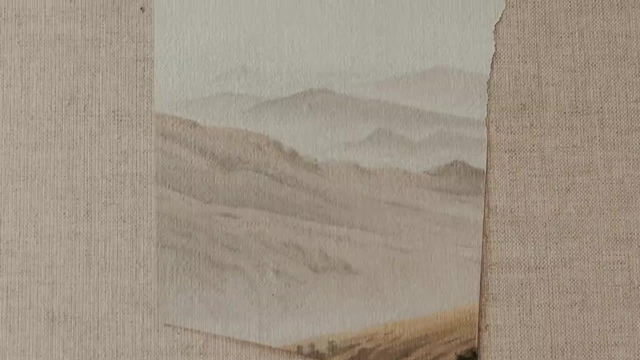 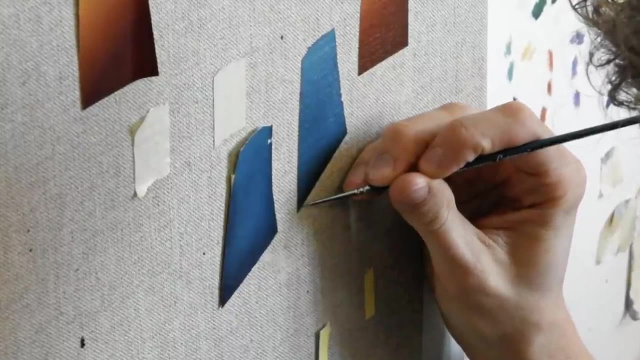 to the canvas. However, there is no masking tape, nor can we find actual small pieces of paper depicting a landscape. Everything has been painted, reinvigorating Tromp-Loy painting in an era in which mimesis and the niche of Tromp-Loy painting seem to be a thing of the past. 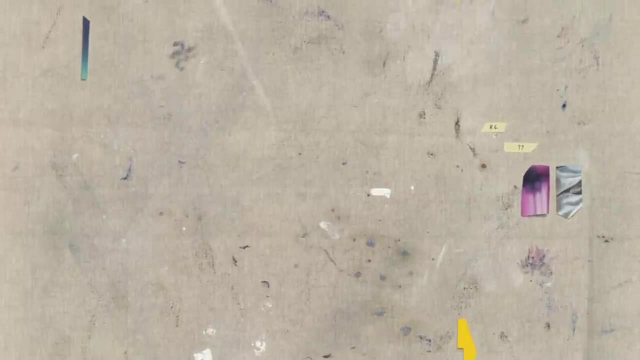 Doing so. Gobben examines the art of painting and finds that it is a thing of the past. Gobben examines the artistic process of painting. He questions the status of painting not only as an image, but also as a process and object. 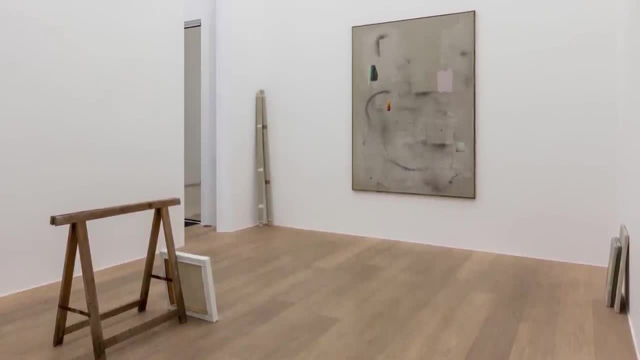 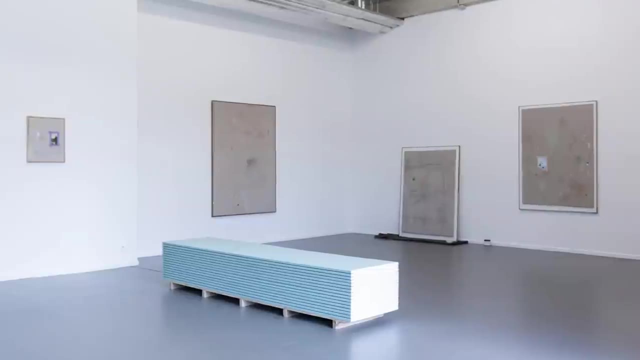 We encounter a similar strategy when it comes to his exhibitions. It seems as if the gallery space is not finished yet and they are still in the process of building the show. Masking tape, unhung paintings or a ready-made decorative sculpture of a pile of drywalls can. 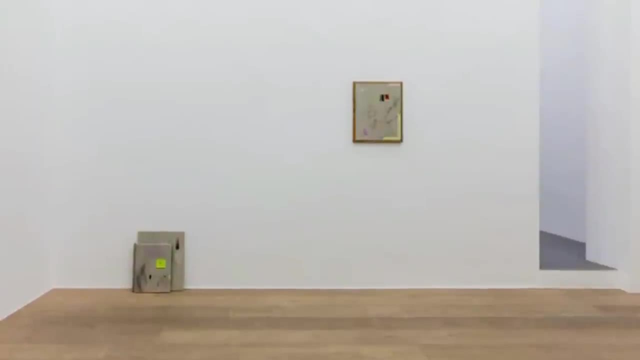 be found on the gallery floor. Ritzit Gobben's works and shows are something different as a result of his work. Gobben's works and shows are something different as a result of his work. As a result, we are convinced he is one of the artists to watch in 2022.. 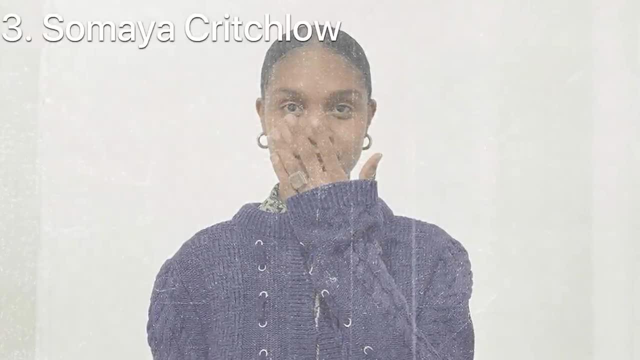 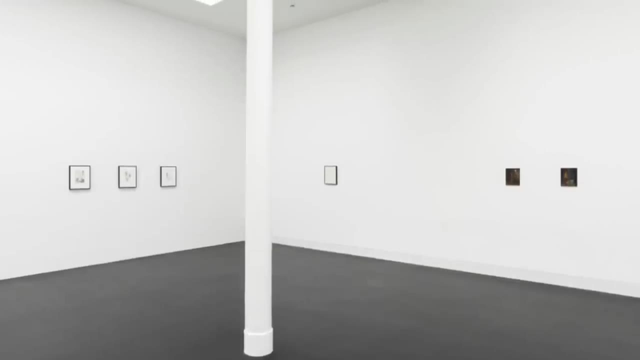 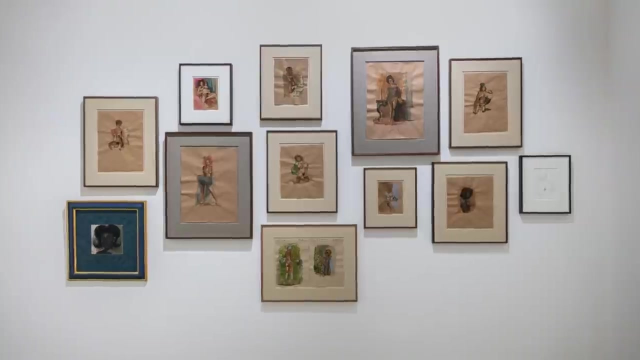 Number 3, Semiah Critchlow. Up next we have the Benjamin of our selection of emerging artists. Semiah Critchlow, born in 1993, lives and works in London. The British artist's figuratively rendered paintings take on the tradition of picture making. One encounters hints of Renaissance. 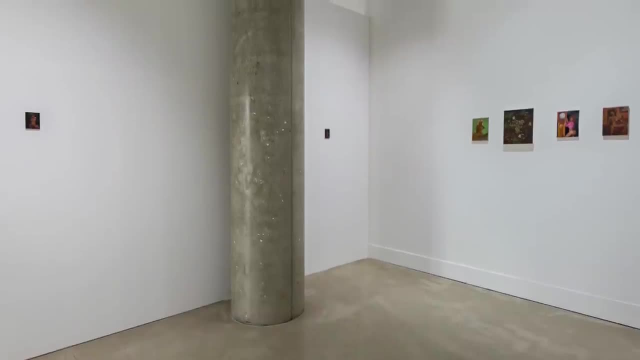 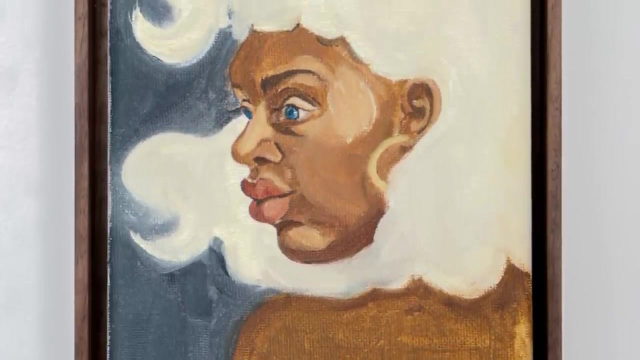 Rococo, Dutch still-life, painting, various traditions and much more in an utmost contemporary manner. The universe of Semiah Critchlow is female, taking on the distinctions between high and low culture, or in class and racial differences. Her intriguing body of works. 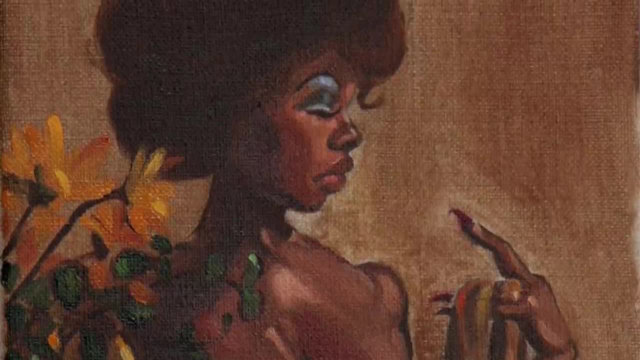 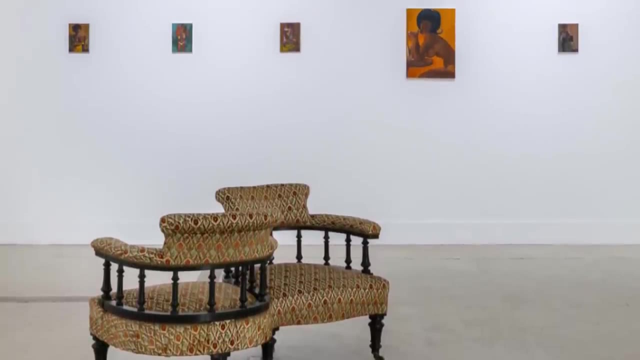 hasn't gone by unnoticed. In fact, Critchlow was one of the fastest-growing artists in 2021, according to the ArtFacts algorithm, and we strongly believe the young emerging artist hasn't reached her peak yet. So watch out for Semiah Critchlow. 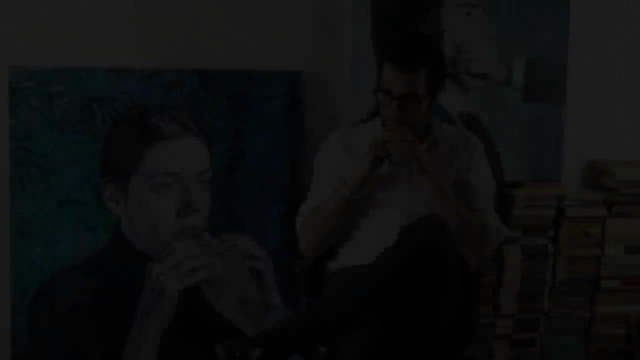 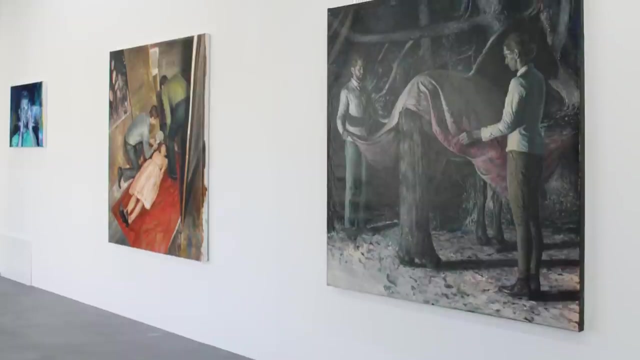 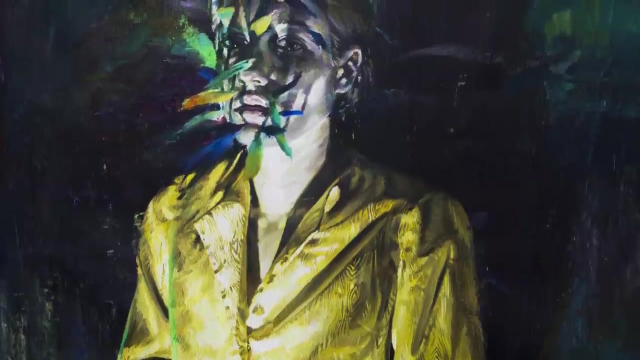 Number 4, Remus Grecu. Our next artist is none other than Remus Grecu. In 2021, we had the absolute pleasure to work with the Romanian artist for his solo show at our Exhibition Space CHI Gallery. From all the artists we have met and seen throughout 2021,- 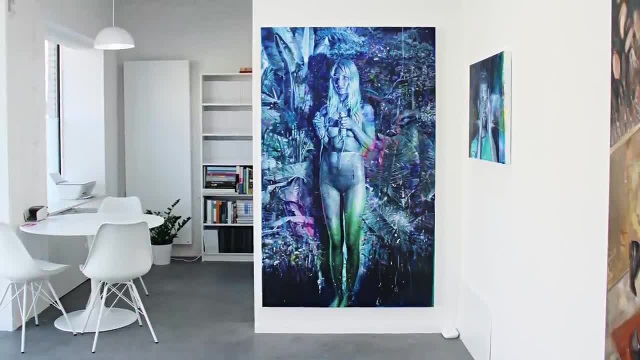 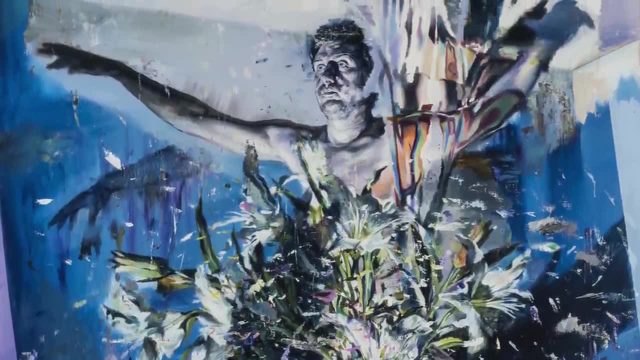 Grecu is the painter we are most convinced of to be destined for greatness, especially after such a highly successful year. Born in 1976, Remus Grecu is one of the most famous artists in the currently resides and works in Bucharest. He is best known for his dazzling figurative paintings. 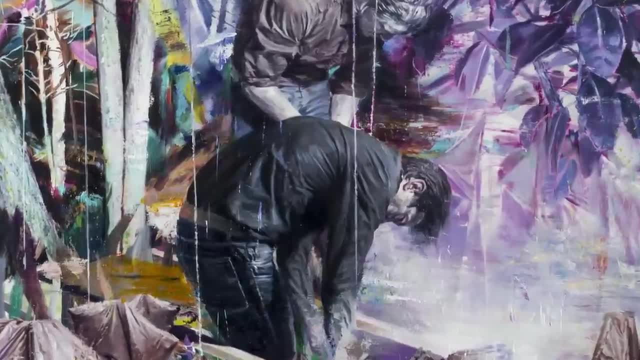 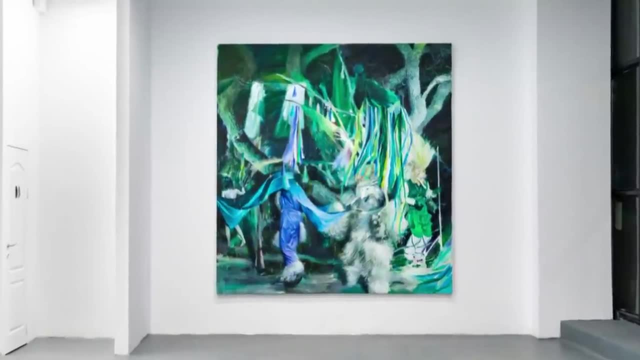 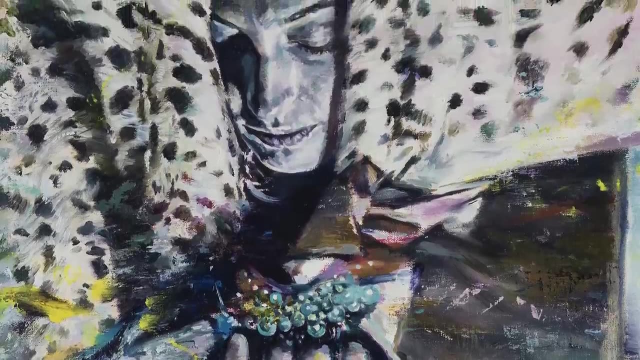 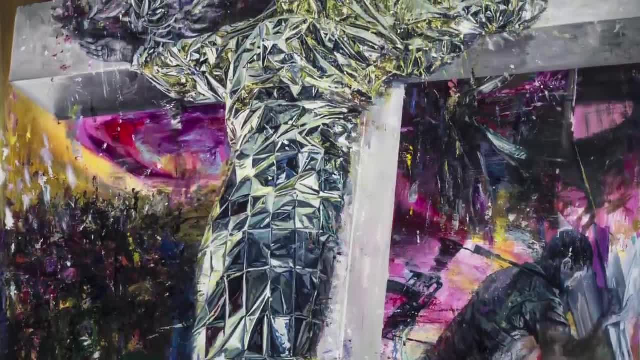 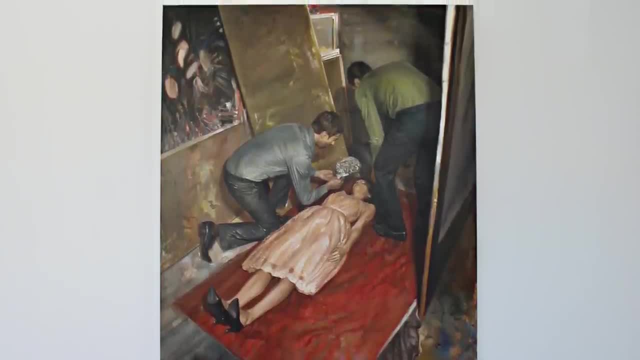 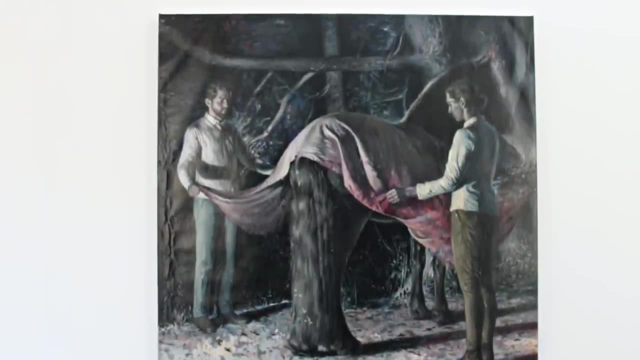 Grecu is set for another terrific year in 2022.. For any further inquiries on Remus Grecu, we are happy to assist you and remain at your full disposal, So do not hesitate to request a catalogue with available works. 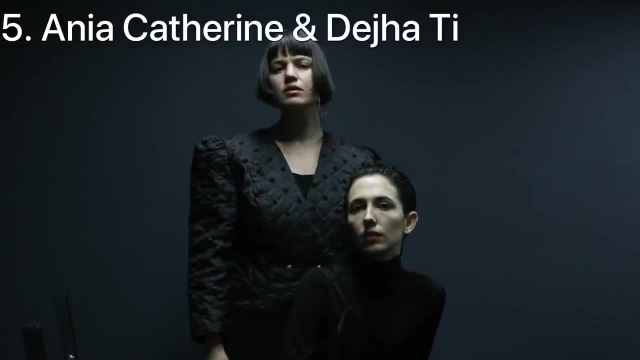 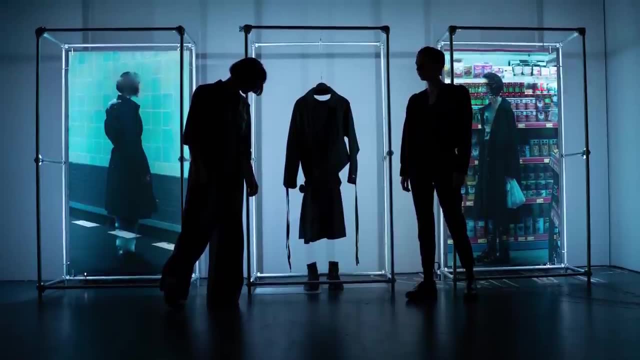 Number 5.. Ania Catherine and Deja Tai. Next we encounter our special guest Grecu. He is a great artist and he is a great artist. Deja Tai and Ania Catherine, The award-winning duo from Los Angeles, currently resides and works. 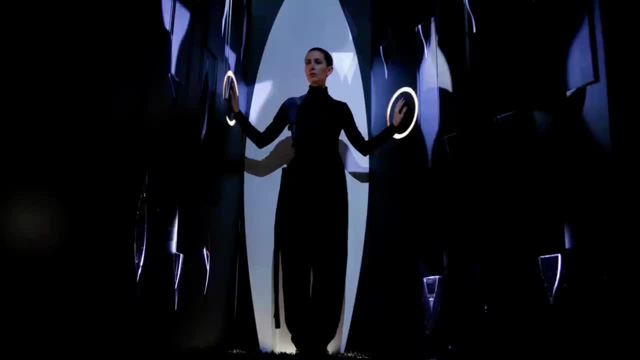 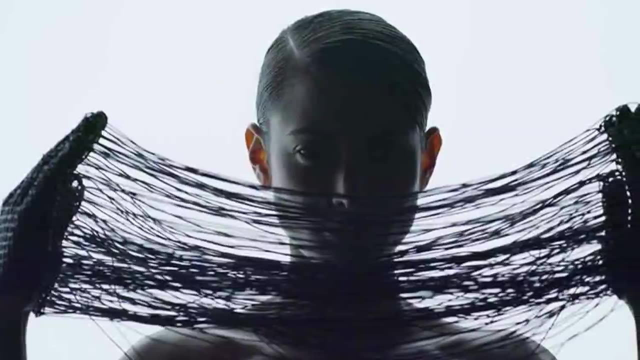 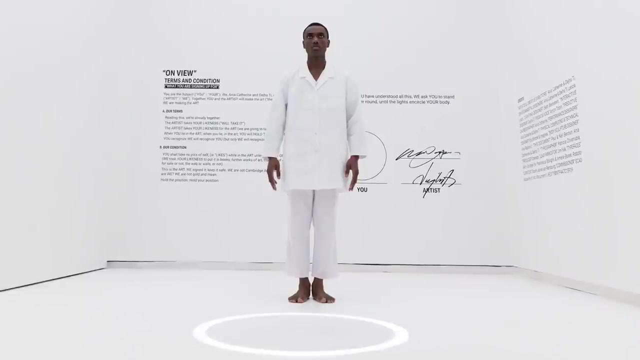 in Berlin, Germany. Tai and Catherine distinguish themselves with their unique and project-based artistic practice, creating immersive experiences, guiding the viewer into an idiosyncratic world, questioning socio-political issues by manner of interactive installations. The duo of conceptual artists create immersive digital artworks in the form of large-scale 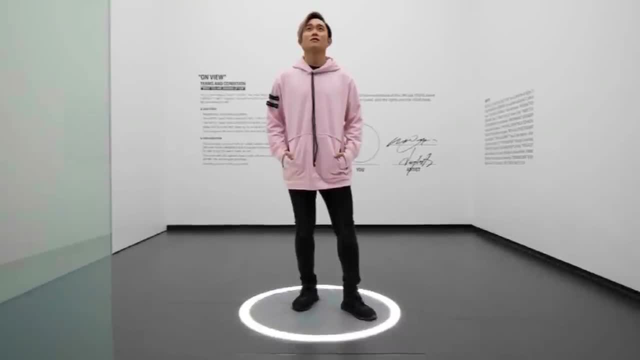 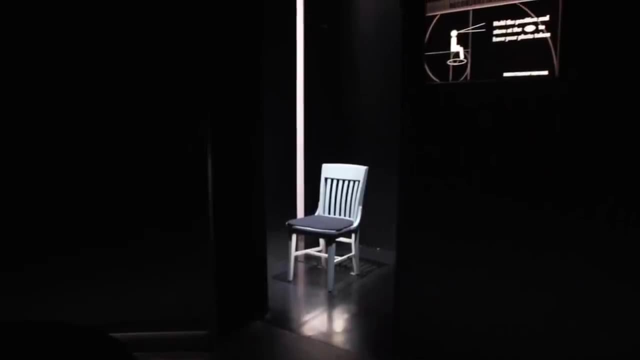 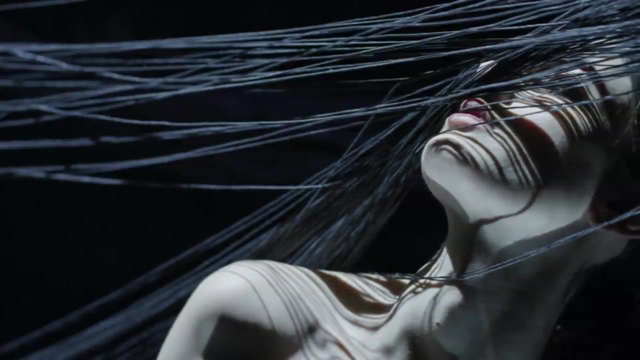 installations. Whereas often the new possibilities of digital in art seduce the viewer by manner of presenting a spectacle, Deja Tai and Ania Catherine take a more refined and subtle approach when it comes to immersion, producing a feeling instead of a spectacle, By taking on thought-provoking subjects. 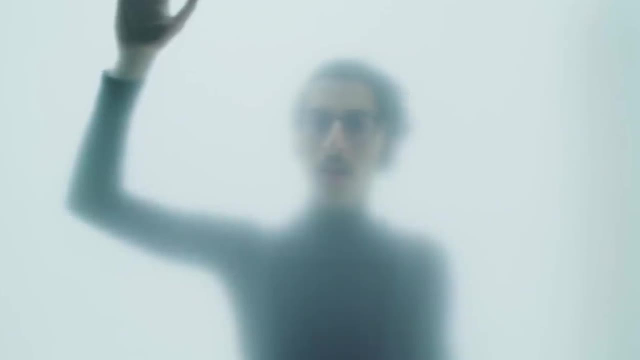 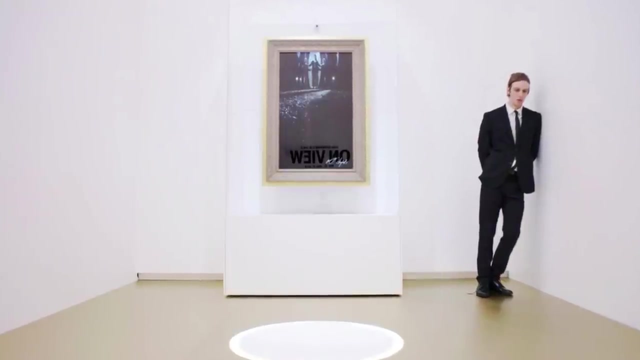 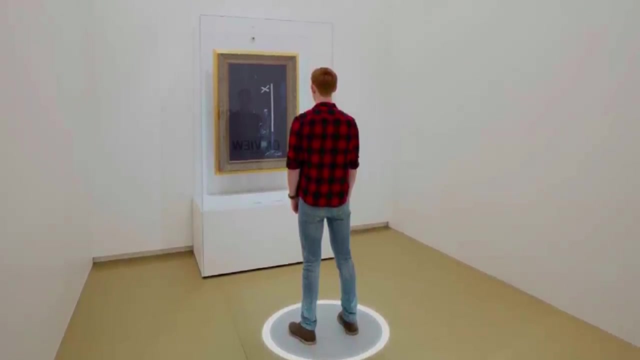 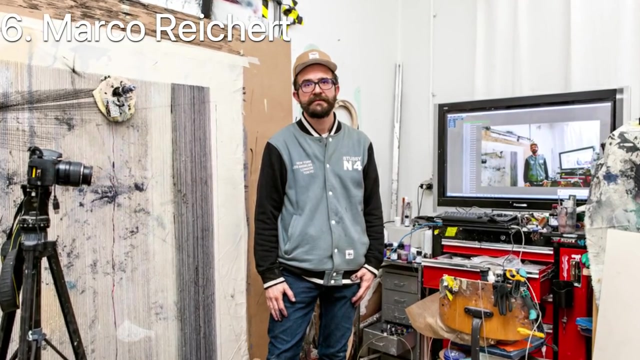 in a multidisciplinary manner. the duo is set to take the European continent by storm, having moved very recently across the Atlantic. As a result, in 2022, we are following their projects with the greatest interest: Number 6. Marco Reichert. Born in 1979,, Marco Reichert is a German artist working. 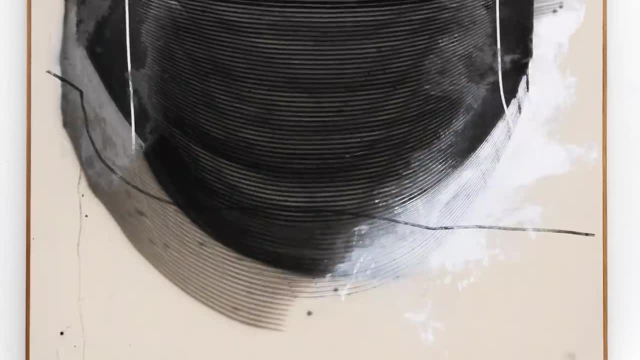 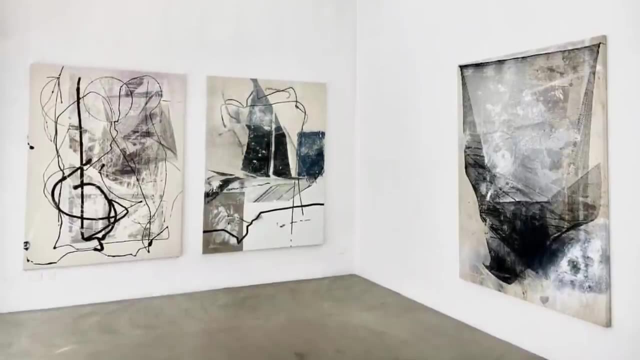 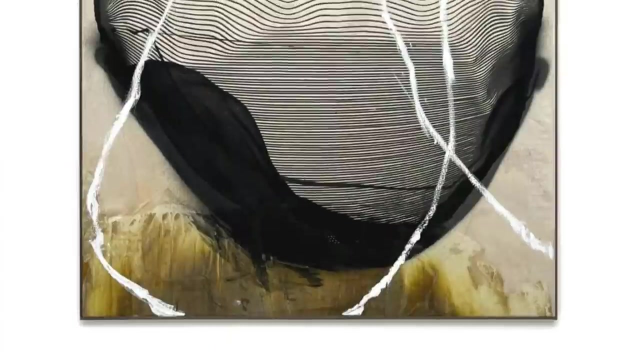 and residing in Berlin. The aesthetics of Reichert's contemporary paintings have convinced art collectors strongly throughout 2021.. As a result, Marco Reichert is one of the artists to watch in 2022, as his career seems to be in a moment of acceleration. The unique technical 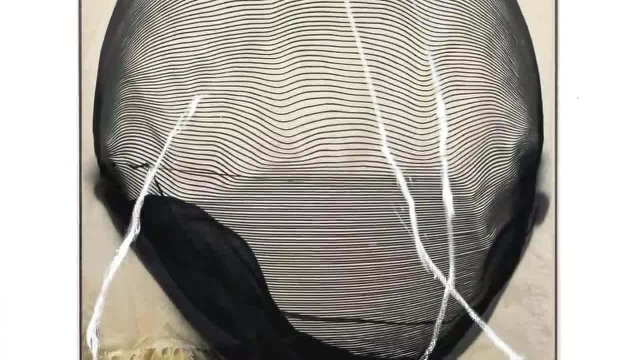 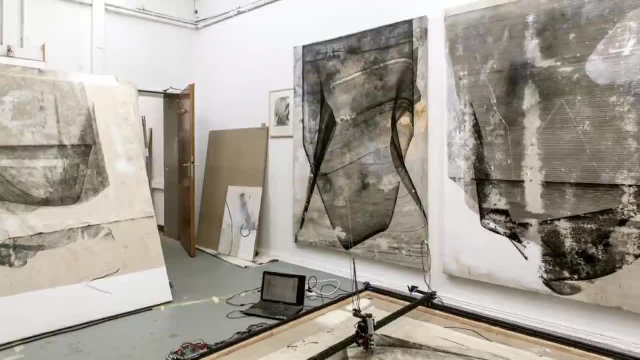 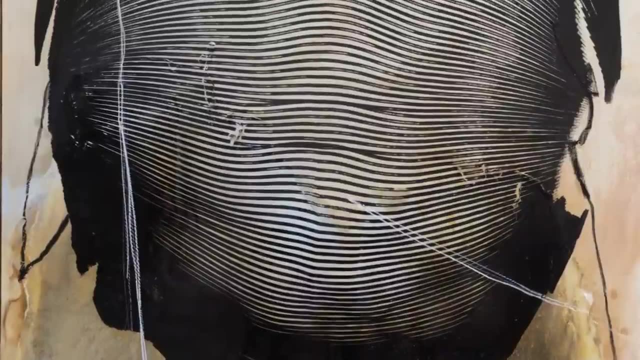 procedure of Reichert's characteristic paintings consists of a very sophisticated and unique creative process, implementing machinery using computer technology. Doing so, the German painter hovers between graffiti, computer art and traditional painting, The contrast of the mechanical character of his black lines and the expressive interventions of the artist. 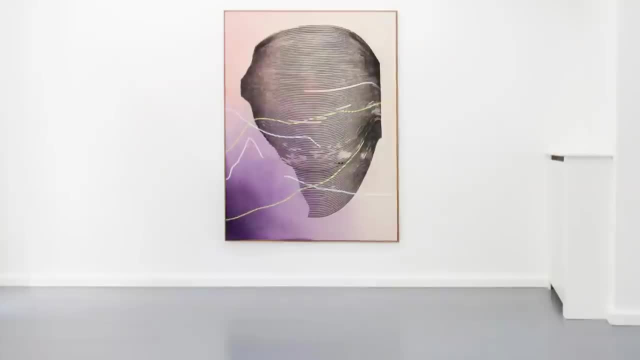 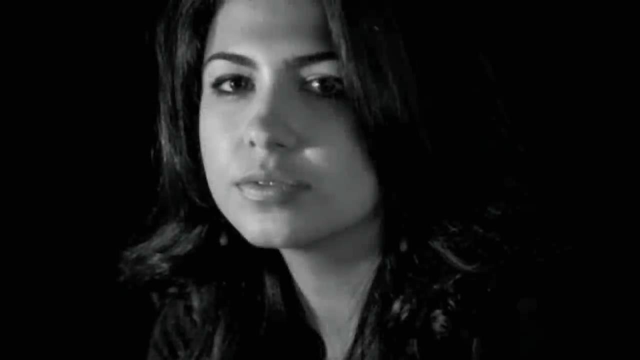 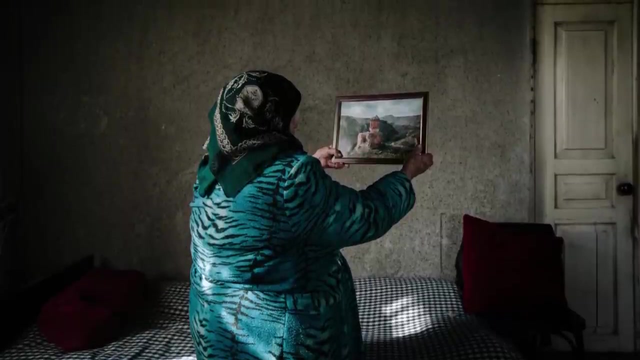 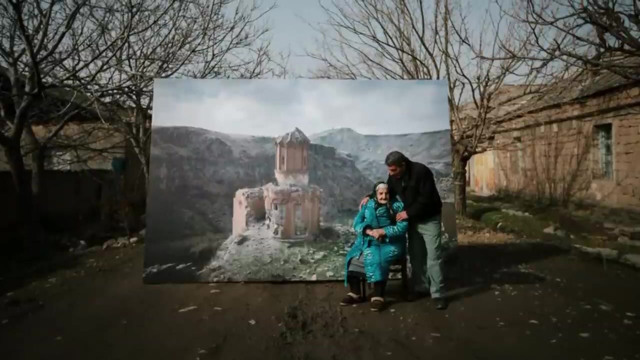 result in an uncanny tension and play-off balance. Therefore, in 2022, watch out for Marco Reichert, Number 7. Diana Markozian: We conclude our list with none other than Diana Markozian. Born in Moscow in 1989, the Russian-American photographer of Armenian descent has been on the rise convincingly, In particular ever since publishing her first. 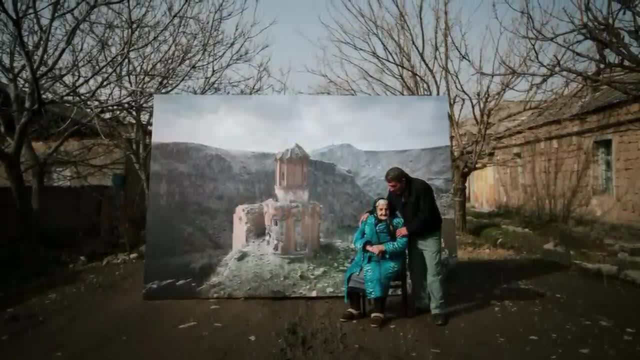 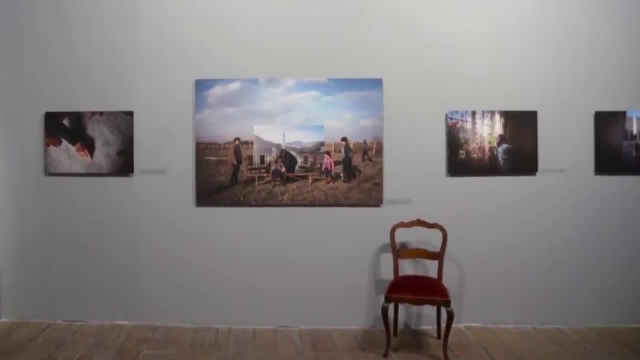 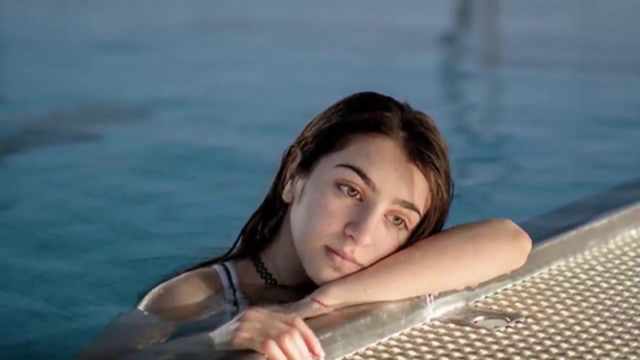 monograph Santa Barbara, published by Aperture in 2020, her career has been carrying a lot of momentum into the new year. Her fine art photography is marked by an ongoing exploration of memory and place. Markosian's artistic practice is marked by an interdisciplinary process. Doing so. 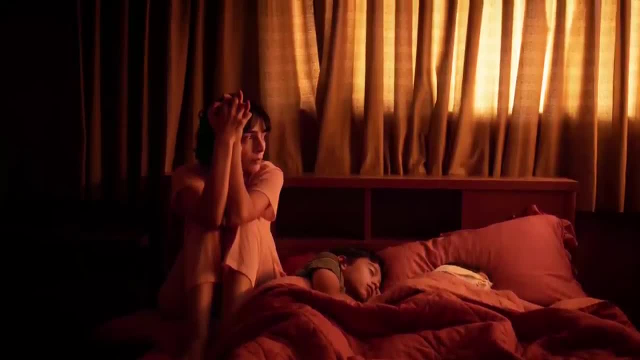 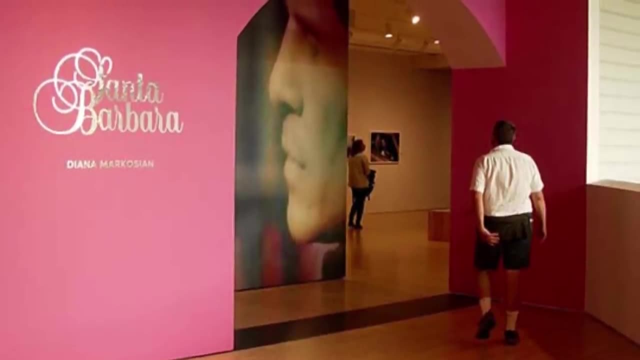 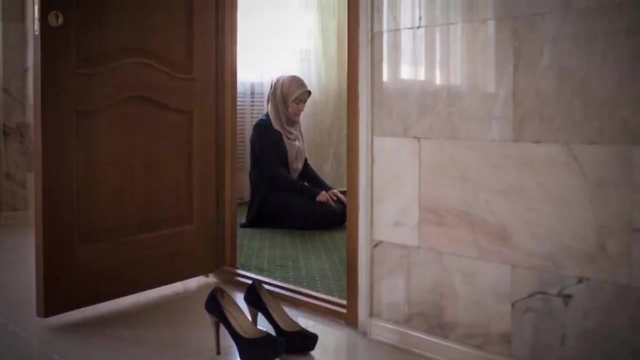 Markosian encompasses video, photography, drawing and historical ephemera throughout her creative method, With shows at the San Francisco Museum of Modern Art in 2020, and the International Center of Photography in New York last year. Markosian is one of fastest growing artists in the world.